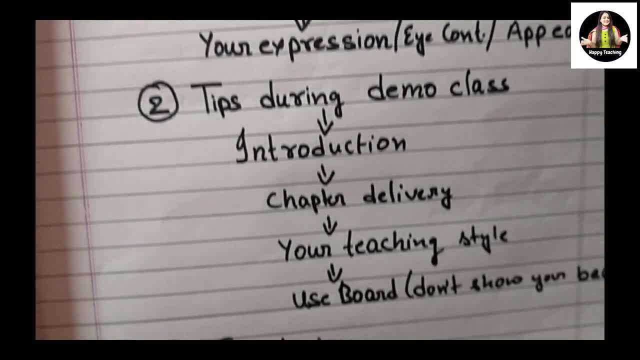 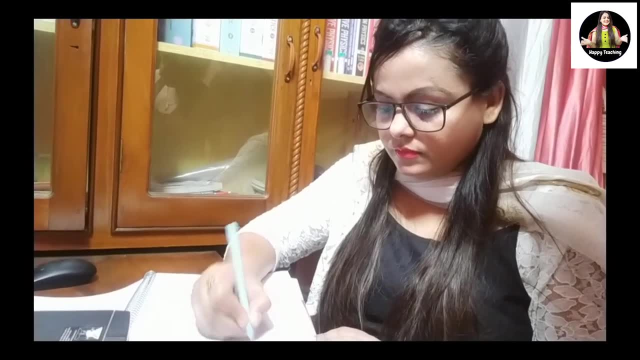 So here are the tips, which I will explain one by one in this video. Let's start with pre-demo preparation. Now, what is pre-demo preparation? So let's start with the pre-demo preparation. before going to demo class, do pre-demo preparation for that. what you have to do is choose your. 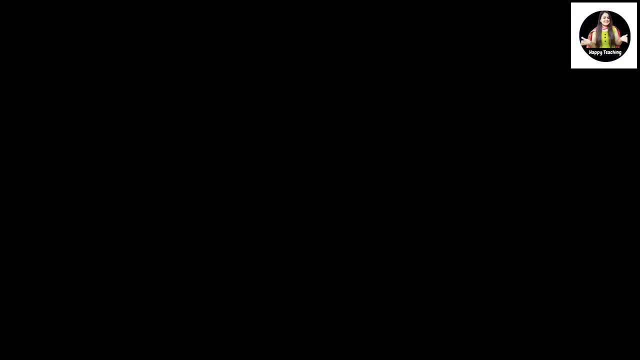 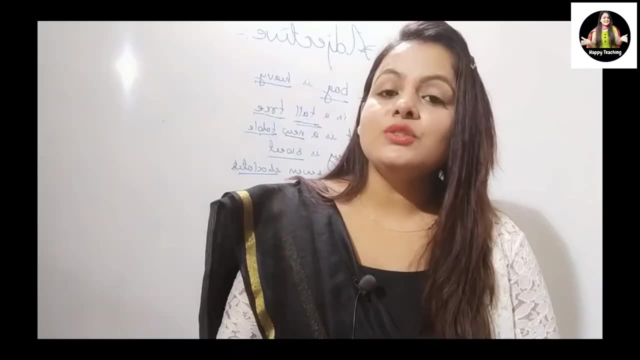 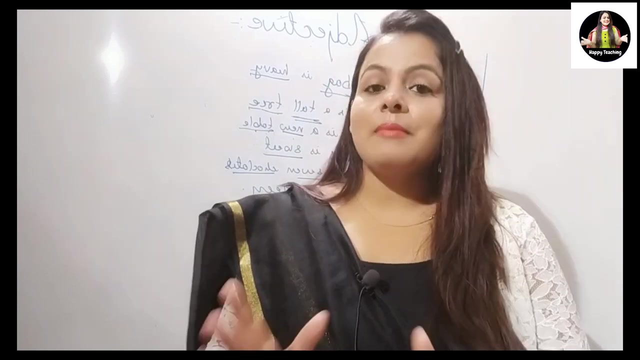 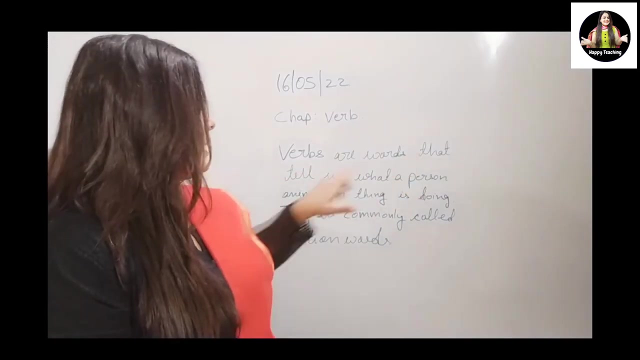 subject and in that subject, what topic you're going to prepare. select it always. choose the topic which is your favorite one and in which you have a very good command, without hesitation. you can explain and you should have enough knowledge on that. next. after that, what you have to do is practice: same topic. take piece of chalk or marker, stand in front of the mirror. 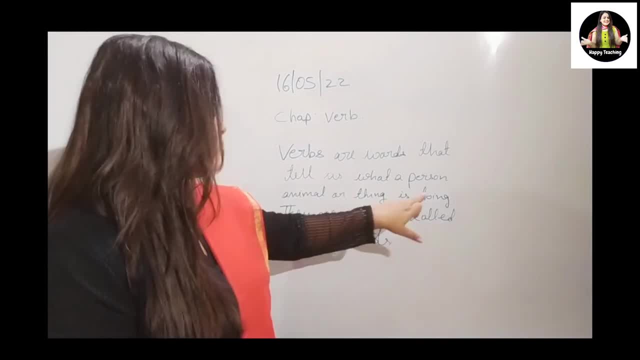 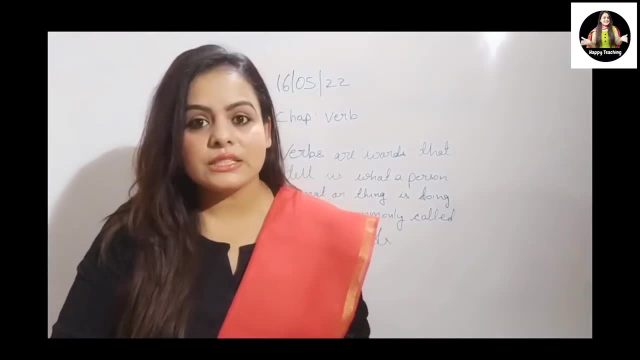 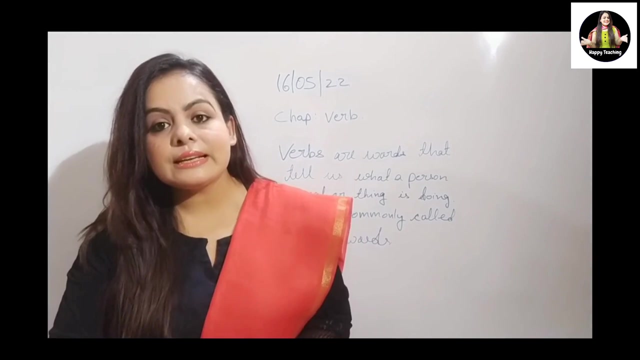 or in front of anybody you feel like. for practicing you don't need any person, just assume that in front of you you have student or interviewer. okay, like in front of me now nobody is there, but just i'm assuming many teachers are there and i'm giving training to them. so in the 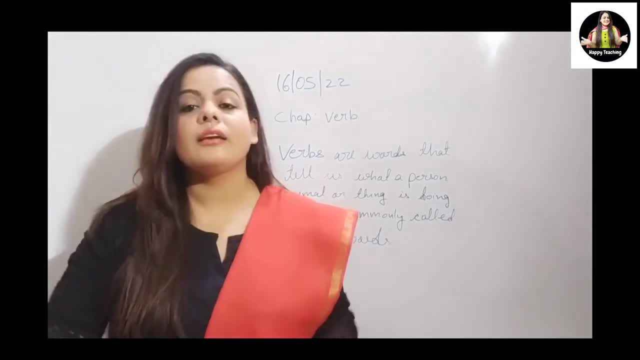 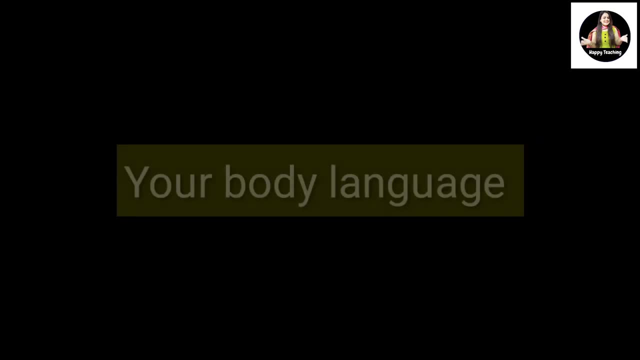 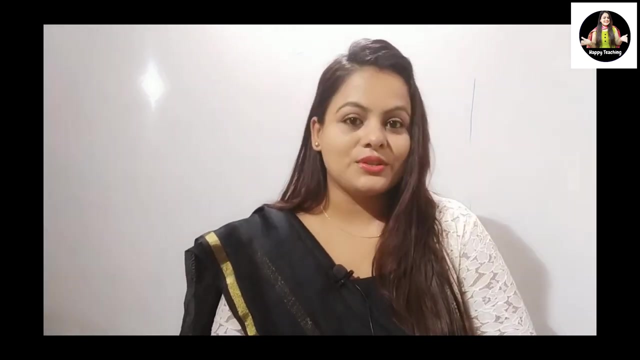 same way practice. you can also use the phone to record your demo session. practice will give you more confidence. next, while doing practice, your body language, your communication skills, play very important role for that. use simple and easy language in which your children feels comfortable. our body language speaks a lot about our personality. 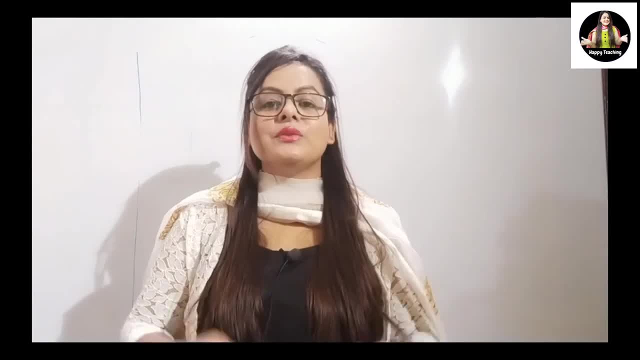 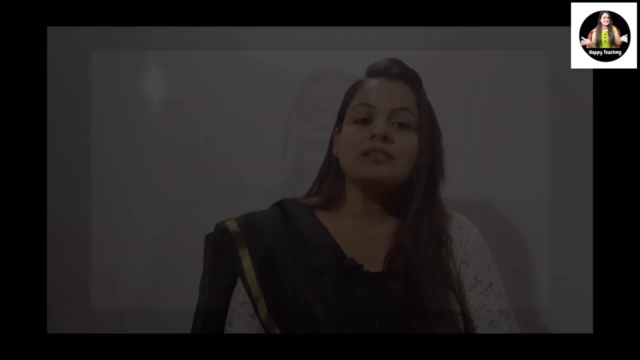 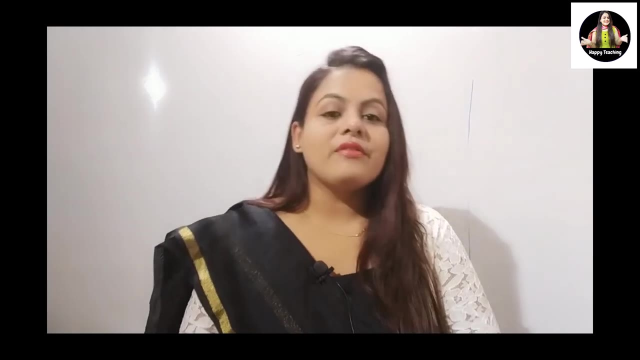 so always relax cool, pleasant face with gentle smile and also maintain proper eye contact to each and every student. don't just give your attention to one who is very active or very good in your class. you are a teacher. that kind of body language you have to maintain. next one is: 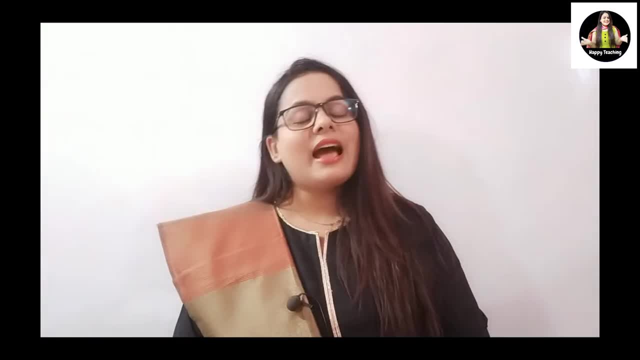 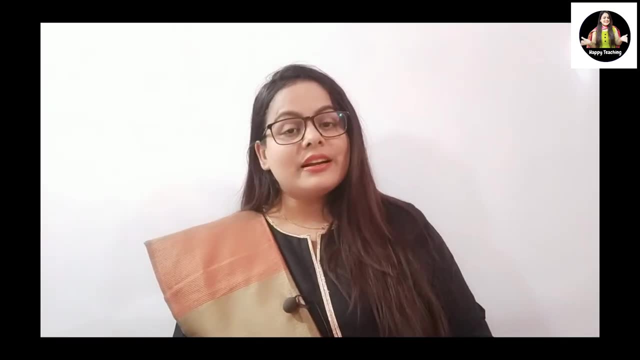 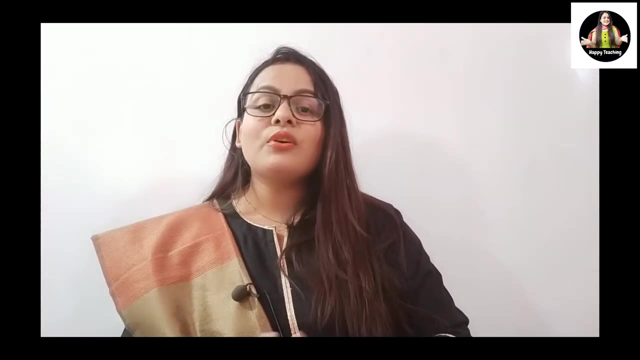 appearance. your appearance should be always decent, always wear decent color, decent dress and also it depend on the school where you're applying. like if you're going for international school, observe the custom of that school and dress up yourself according to that. so these are the things which comes under your pre demo preparation. now let's talk about daring your demo class. what? 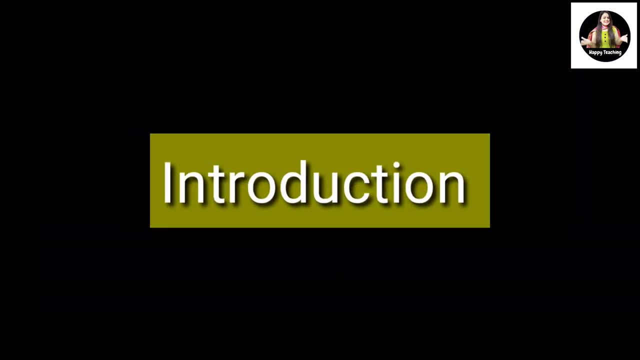 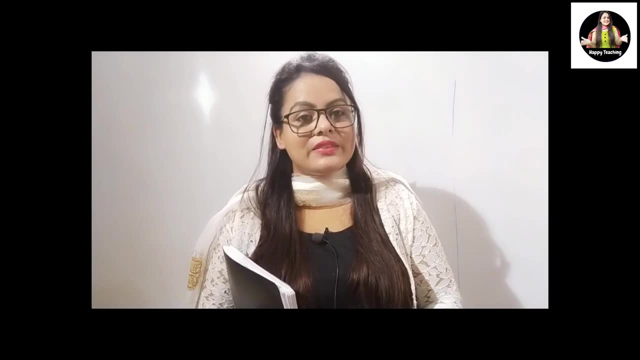 are the things you should keep in your mind. okay, introduction: introduce yourself before you start your class. be cool and confidently introduce yourself, like how I'm giving my introduction hello class. my name is Maru and today I am going to take your geography class. okay, please check out. 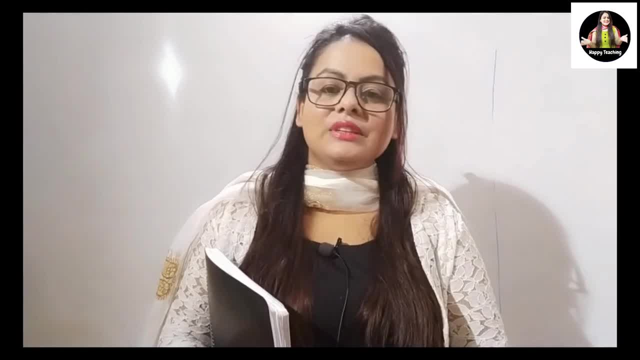 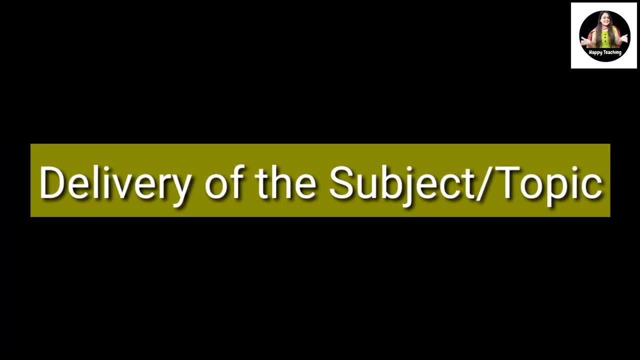 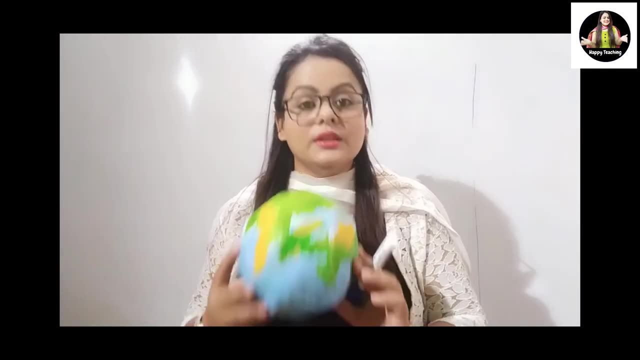 your book, page number 17 and the name of the chapter is inside our earth. okay, now a After introduction. what comes is delivery of the subject. okay, Don't rush with the topic. Explain point to point, Take your time, Take student time to understand. 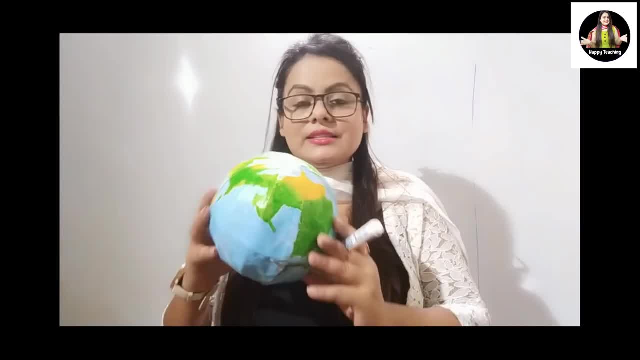 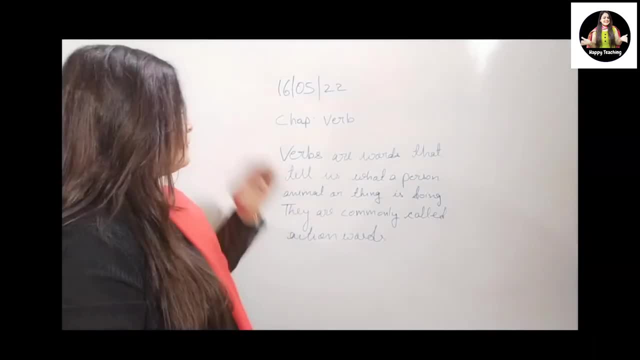 Let them understand the topic first. okay, Step by step. First, give introduction of the topic, Define it in few sentences and then go depth, but slowly, slowly, okay. Next, while explaining the topic, your teaching style play an important role. 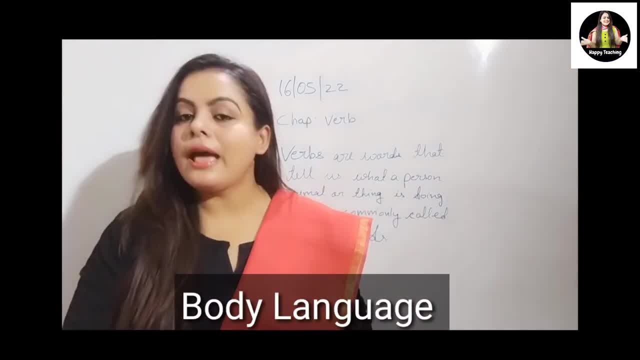 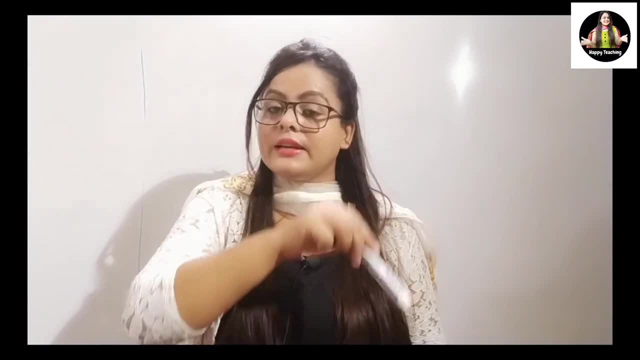 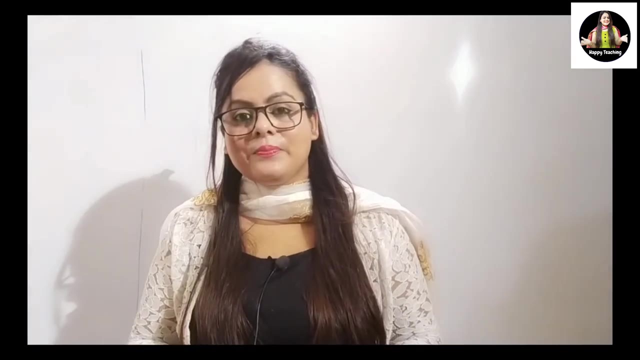 How confidently you are explaining your body language, your ways to explaining the topic really matter. So use your hand, your board, TLM or anything you feel like to use to make your children learn better. okay, So at this particular moment, don't overthink about the interviewer. 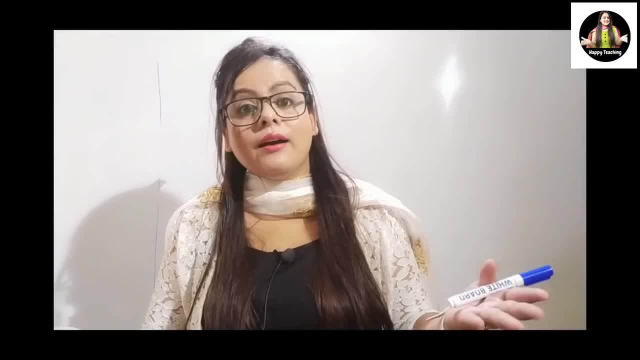 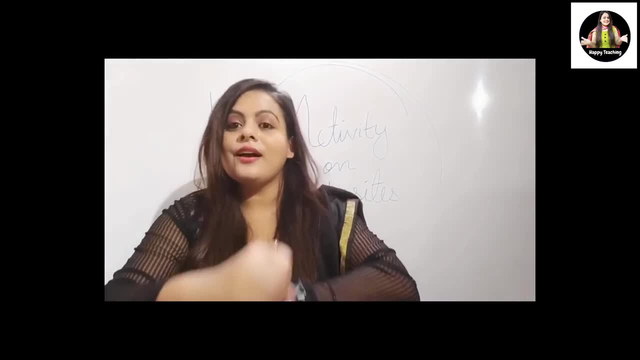 Just focus on your explanation style. Your motto is to make your student understand and grab their attention during your class. okay, When you yourself interact, Enjoy your teaching People around you. they must enjoy your teaching. okay, Now, next is use board. 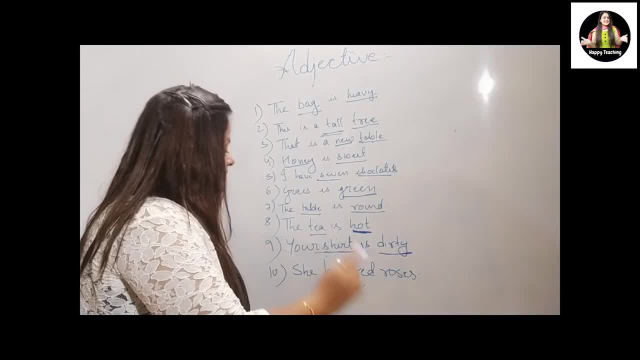 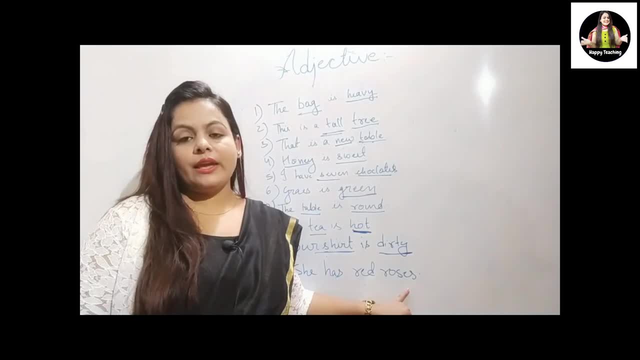 Sometime, due to fear or overthinking, you forget to use board. Using the board is very important, So don't give chance to the board member that you have not used the board. This will be a drawback. So at least to write few things for explaining your topic, just use it. 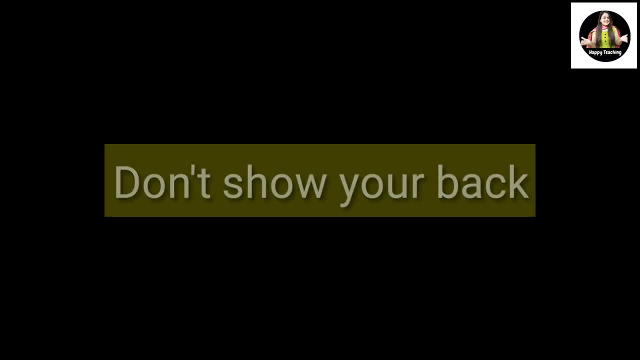 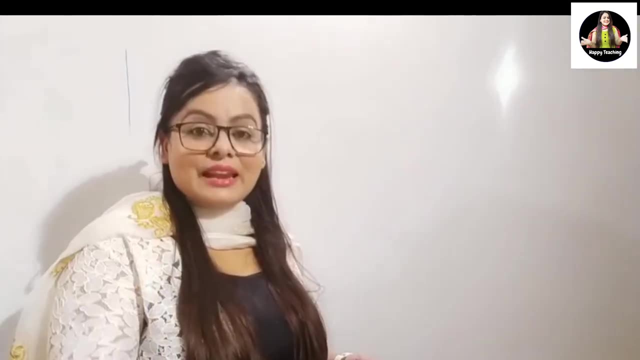 Next, while using board, don't show your back. Never do this. This is blunder in teaching field. When you are writing, this is the right position. Don't give any chance to the interviewer that you don't know how to use the board. okay. 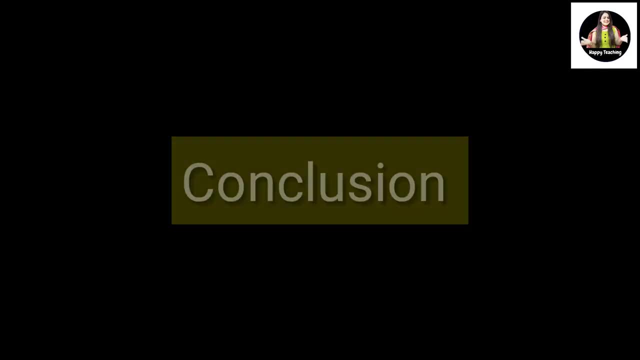 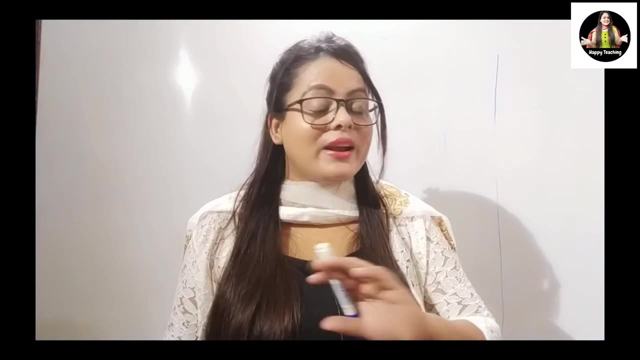 Lastly, conclusion: How should you conclude the chapter or topic? Revise it With student, just wrap up the topic. in short, Just conclude it by asking some questions and doing some interaction with the children, Like hope. the topic is clear. 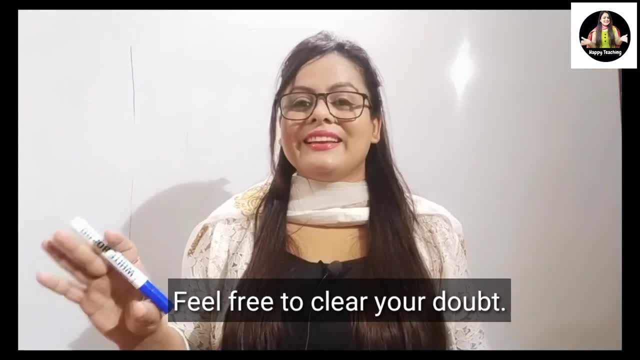 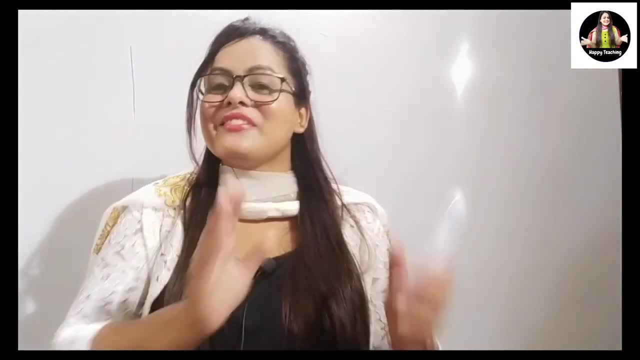 Did you understand? Is there any doubt? Feel free to clear your doubt. It means that you are giving Your student a chance to clear their doubt, if they have any. because they may have some doubt, Okay, give them freedom to raise the doubts and clear it politely.